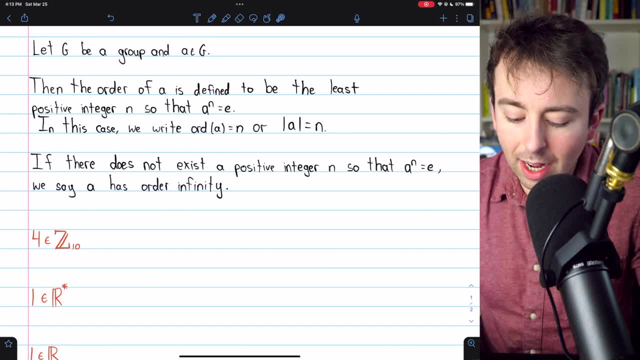 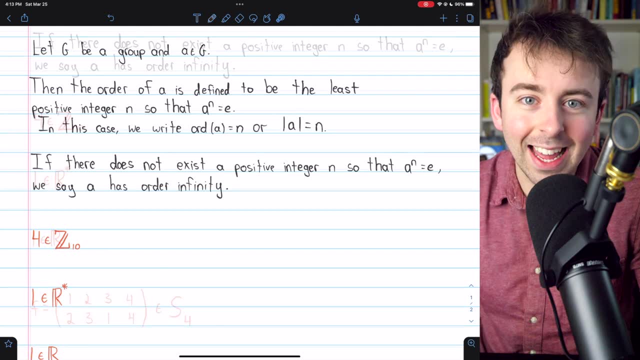 And of course, if there does not exist such a positive integer, we say that the element has order infinity. It doesn't matter how many times you compose it with itself, you're not going to get back to the identity. All right, here is our first example. The number four, as an element 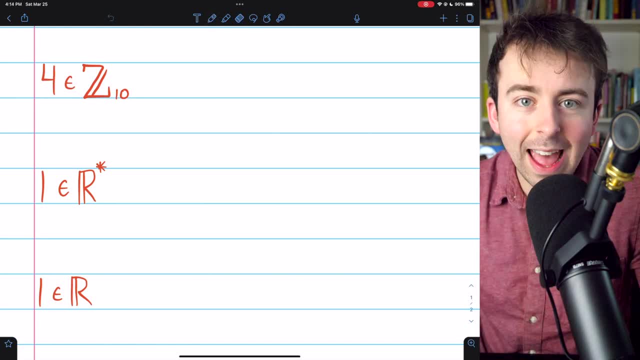 of the additive group of integers mod 10. What is the order of four? Well, here we're talking about addition. So instead of using this notation of four to the n, it would be more appropriate to use the notation of n times four, because this is representing repeated addition. So how many times do we have to add four to itself to get to the identity, which is zero? That's the question. 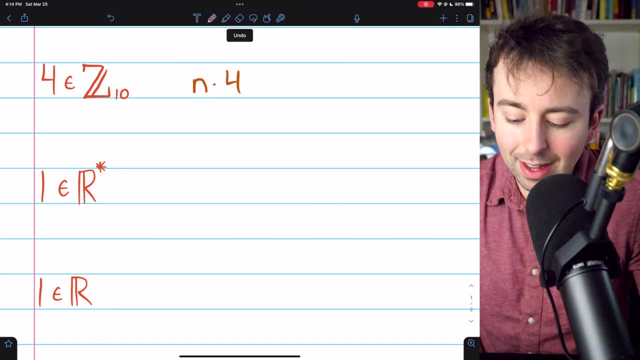 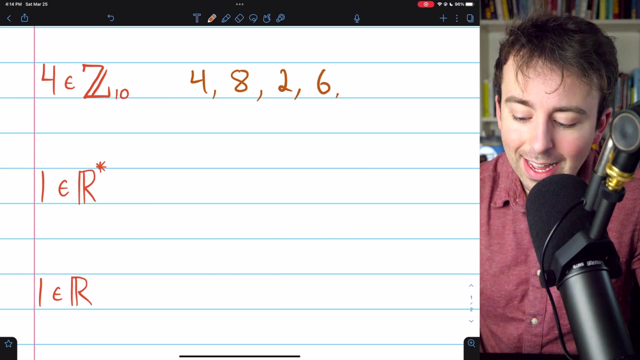 What's the smallest positive integer? So that this is equal to zero. Well, if we have one times four, that's just going to be four. If we have two times four, that's going to be eight. Again, this is all mod 10. And then three times four is 12. Mod 10, that's two. Four times four is 16. Mod 10, that's six. And then finally, five times four is 20, which mod 10 is equal to zero. 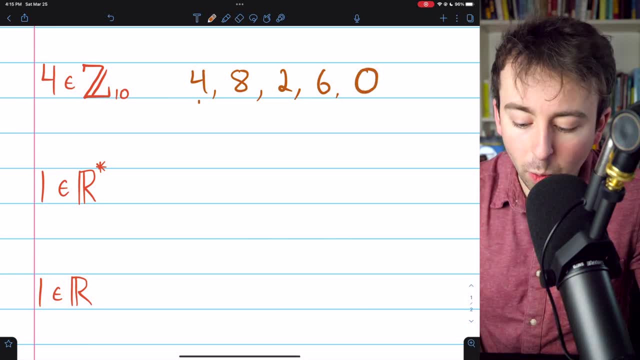 So we saw one times four, two times four, three times four, four times four, and then five times four. That was the least positive integer, five, so that that number times four was the identity. And so the order of four, which we can denote like this, is equal to five in this group. 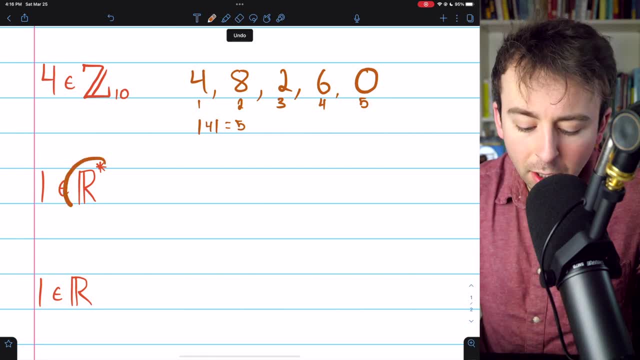 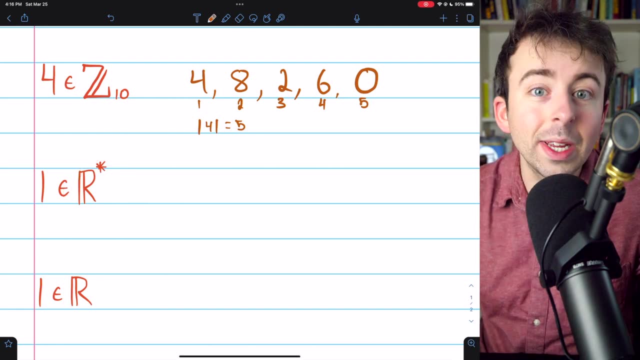 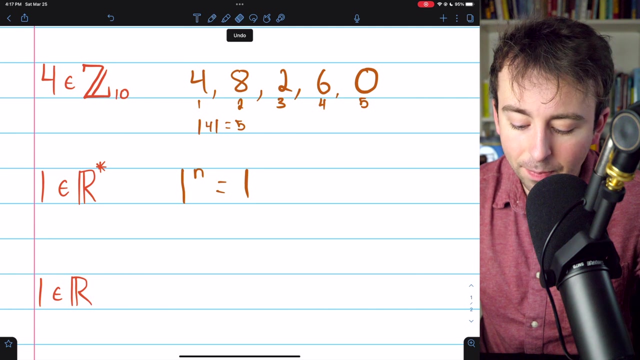 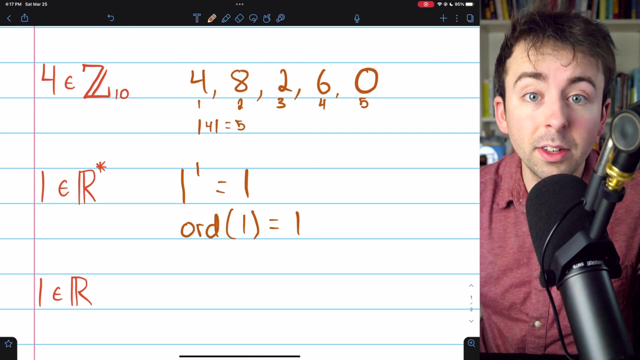 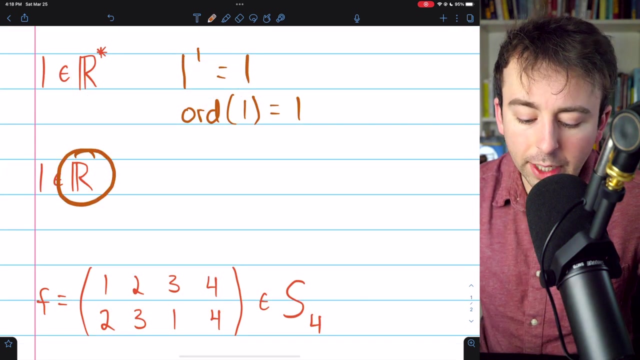 Next, let's find the order of one as an element of the multiplicative group, of real numbers. This asterisk denotes that we are excluding zero, so we can consider this as a multiplicative group. And since we're talking about multiplication, we can use the multiplicative notation. And so we're asking, what is the least positive integer n, so that one to the power of n is equal to the identity? What's the identity? Well, in this case, since we're talking about the multiplicative group of real numbers, the identity is one. And so clearly, the order of one is one. If we make this n equal to one, well, that is the smallest positive integer, and it so happens that one to the one is equal to one. So certainly, the order of one, which we could also denote like this, as opposed to using that magnitude notation, the order of one in the multiplicative group of real numbers is equal to one, because one is the smallest positive integer, such that when we raise one to that power, we get the identity, which is, in this case, one. Saying one a lot makes that confusing, but let me know if you have any questions in the comments. In this next example, we're not removing zero from the real numbers, and so we're talking about the additive group of reals, and we want to find the order of one in this group. So we're asking, what's the smallest positive integer n, so that n times one is equal 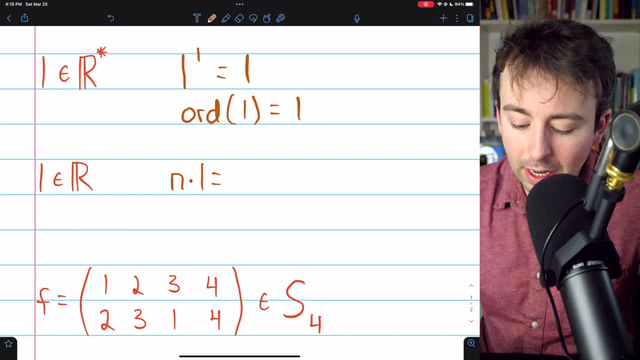 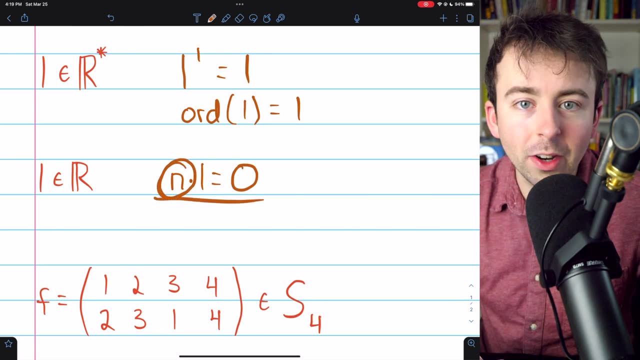 to the identity? In this case, since we're talking about addition, the identity is zero. And in this example, there is no positive integer n satisfying this equation. So there's certainly no smallest positive integer n satisfying this equation. If we take any positive integer n, well, that times one 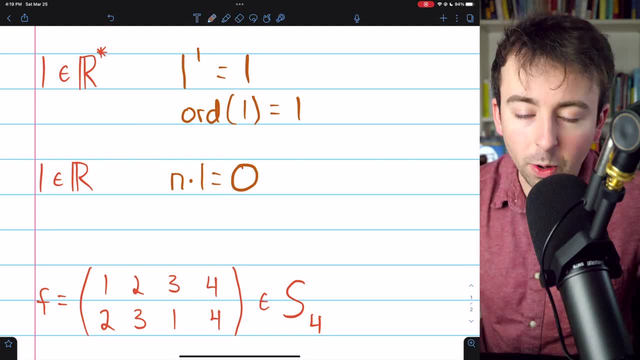 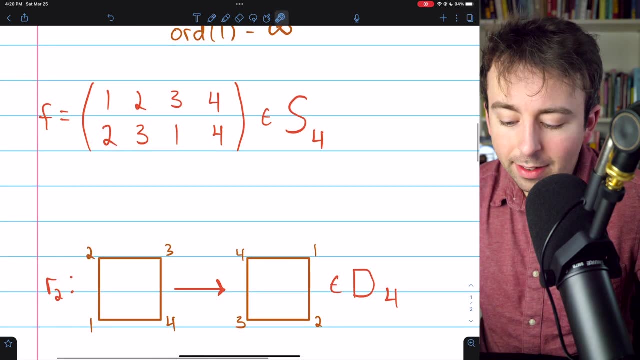 is just going to be n. It's never going to be zero, and so the order of one in the additive group of reals is infinite. All right, in the next example, we're considering this permutation 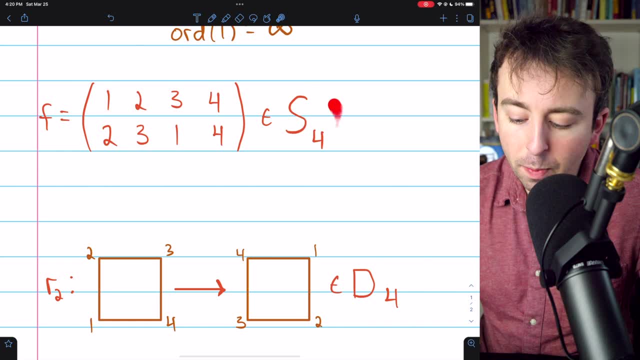 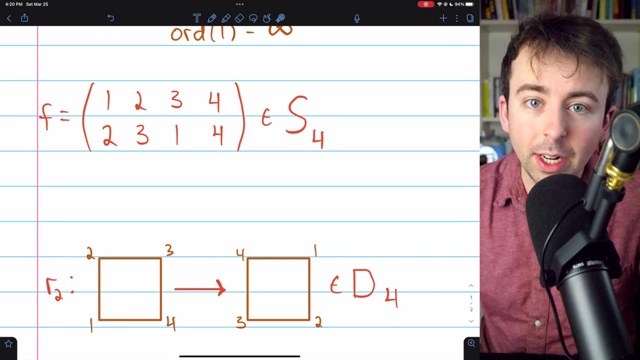 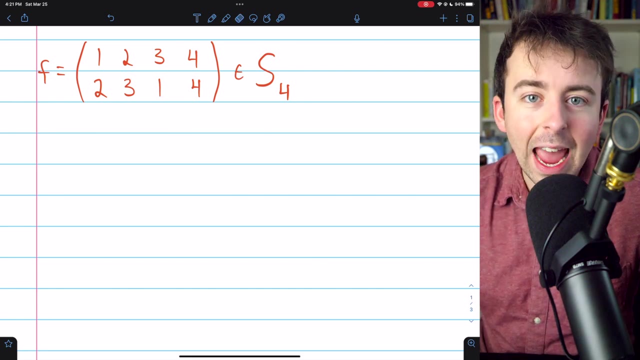 that we're calling f from the symmetric group on four elements. I'll leave links in the description to my lessons introducing permutation groups and symmetric groups if you need a recap on this stuff. But remember, S4 is the group of all permutations on four objects, and the group operation here is function composition. 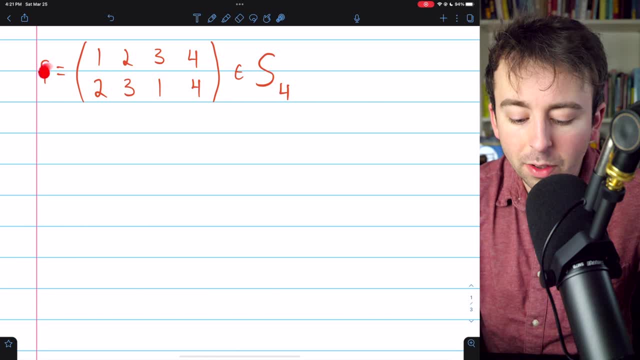 So we're asking, how many times do we need to compose F with itself, which we could represent as F to the n? How many times are we going to have to compose this permutation with itself to get the identity permutation, which we could represent as E? If we compose F with itself a single time, let's see what's going to happen. 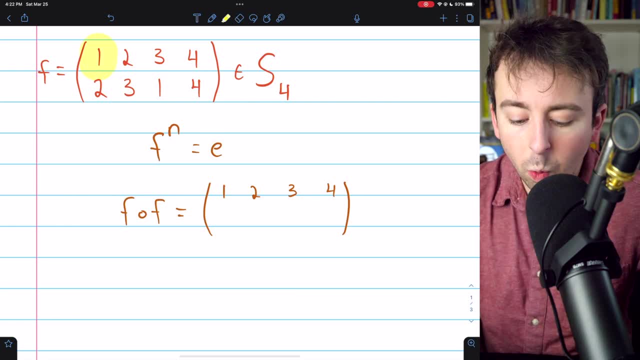 The first instance of the permutation F would send 1 to 2, but then when we compose it with itself, that 2 would get sent to 3. 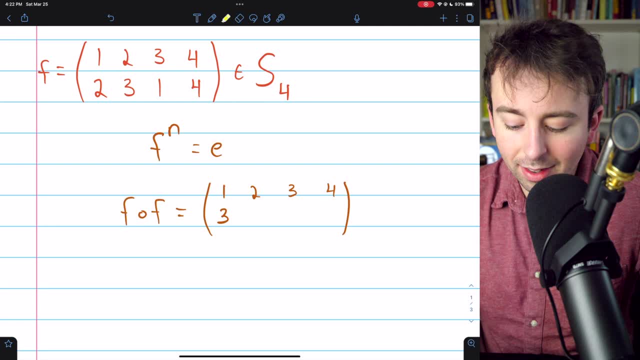 Similarly. The first instance of F would send 2 to 3, but then when we compose it with itself, that 3 would get sent to 1. 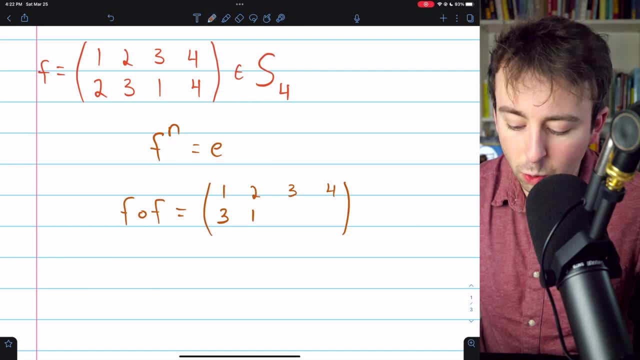 Similarly, 3 would get sent to 1 and then get sent to 2, and then 4 would get sent to 4, and then 4 would get sent to 4 again. And so 4 just maps to itself. 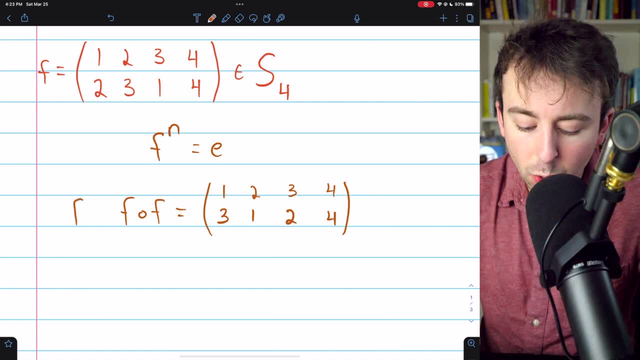 This is what happens when we compose F with itself, which we might write as F to the 2. So. 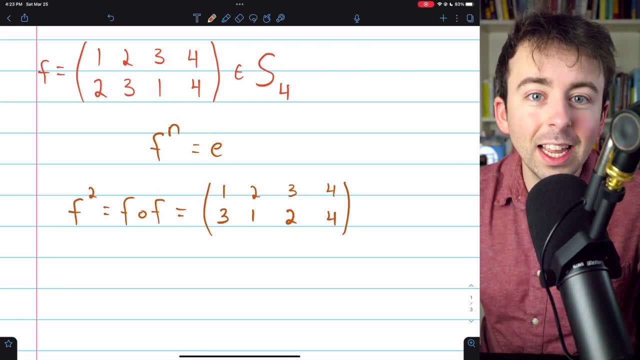 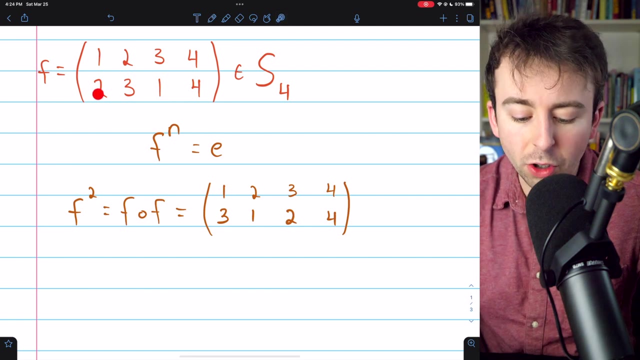 We are asking, how many times do we need to compose F with itself to get back to the identity where none of the elements have actually moved at all? Having seen this example written out, I hope that you can confirm for yourself that the answer to this question is 3. Because 1 will be sent to 2 by the first instance of F, but if we compose it with itself, that 2 will get sent to 3. But if we compose it with itself a third time, the 3 will get sent back to 1. In total, the 1 doesn't move at all. Similarly, the 2 would get sent to 3, but then the 3 would get sent to 1, but then in the third instance of F, the 1 would get sent back to 2. And so the 2 hasn't changed at all. So if we raise F to the power of 3, we are going to get the identity permutation. I'll leave it to you to write that out if you want to verify all of the details. 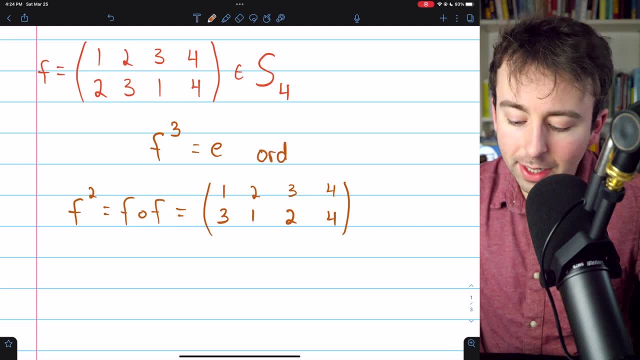 In any case, we see that the order of this permutation F in the symmetric group on 4, elements is equal to 3. 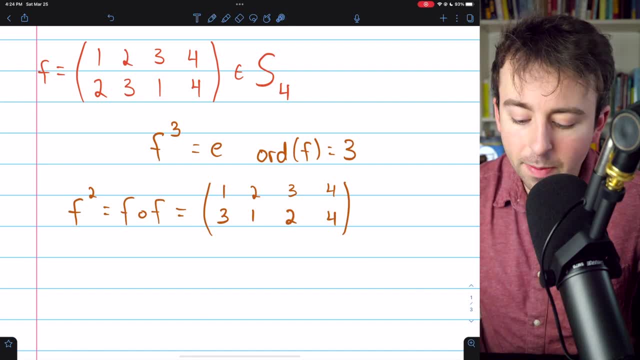 3 is the smallest positive integer, so that F to the 3 is equal to the identity permutation. 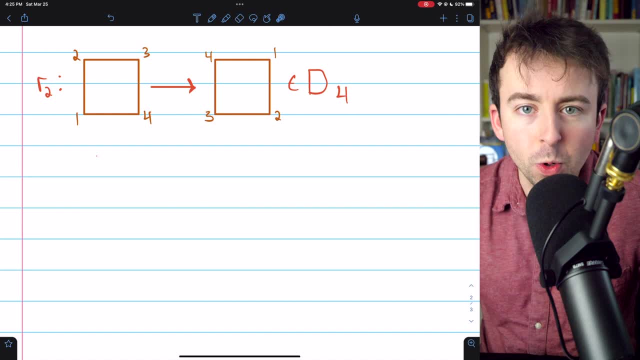 In this example, we want to find the order of R2. This is a 180 degree rotation of a square. It's an element of the dihedral group D4. 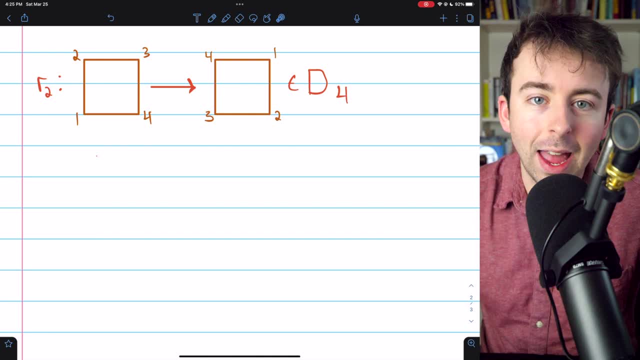 This is the group of all symmetries of a regular polygon with four sides, which of course is... a square. 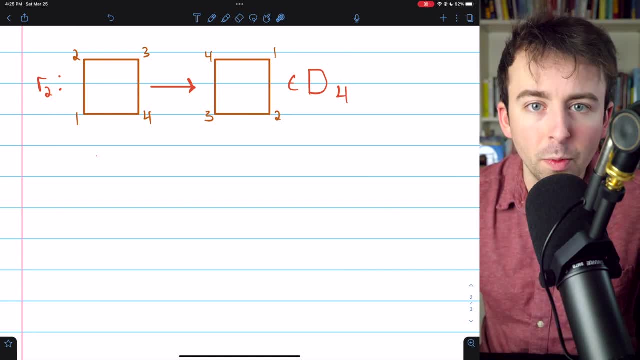 I'll leave a link in the description to my lesson introducing the dihedral groups if you need a recap. I should also mention some authors would denote this dihedral group of symmetries on the square, the 4-gon, as D8, because it has eight elements. But I'm choosing to denote it as D4. Once again, in this group, the operation is composition. So we're asking how many times do we need to compose this rotation, R2, with itself, to get back to the operation? Well, let's start with the identity that hasn't moved the square at all. 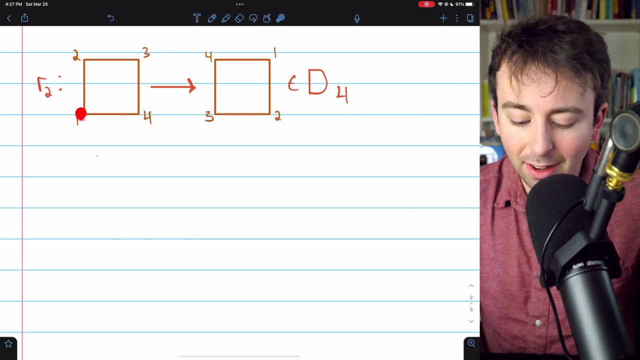 Let me make sure you see how this rotation works. It takes this first vertex and rotates it 180 degrees, right? So one ends up over there, and the two ends up over here after the 180 degree rotation, and the three ends up over there, and so on. 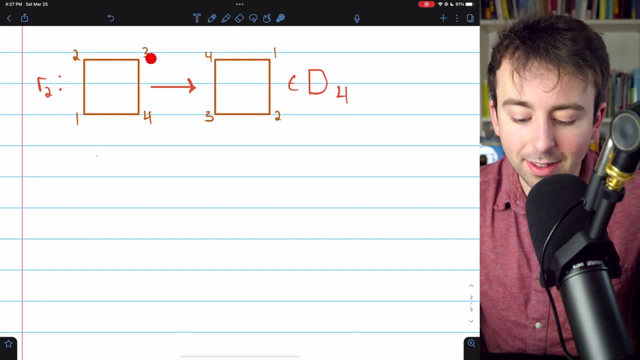 Put simply, each vertex shifts two vertices in the clockwise direction, like the 4, 1, 2. It shifts to that top. That top left corner. All right. Let's try composing this rotation with itself and see what we get. 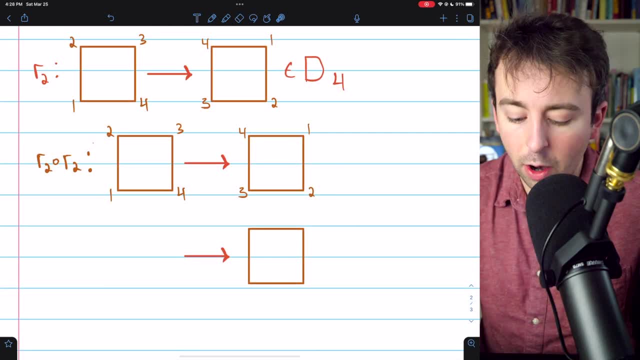 The first instance of R2 we see just moves the square. We already wrote that. That's the definition of the rotation. 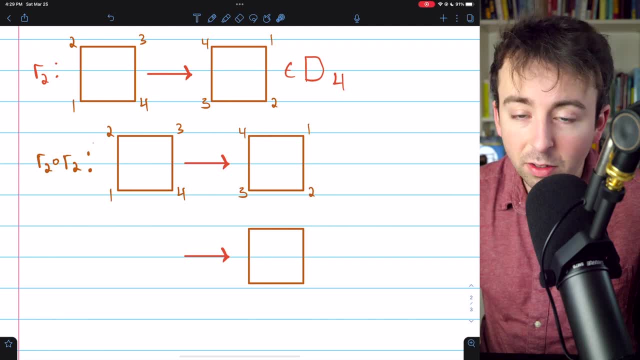 But now, what if we apply that rotation to the end result? So we're composing it with itself. We are doing a 180 degree clockwise rotation of this already rotated square. 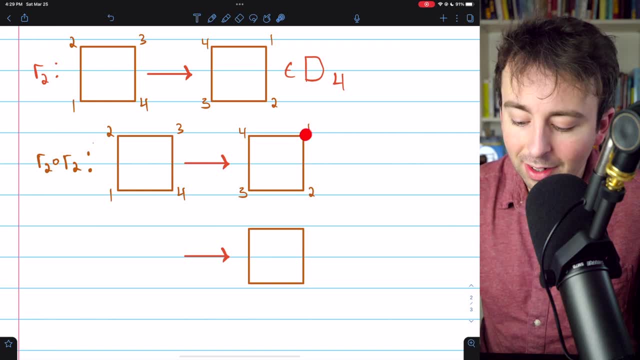 Well, if we do that, then let's focus on the 1 first. It's going to do a 180 degree clockwise rotation. It's going to move two vertices in the clockwise direction, and it's going to end up over here.